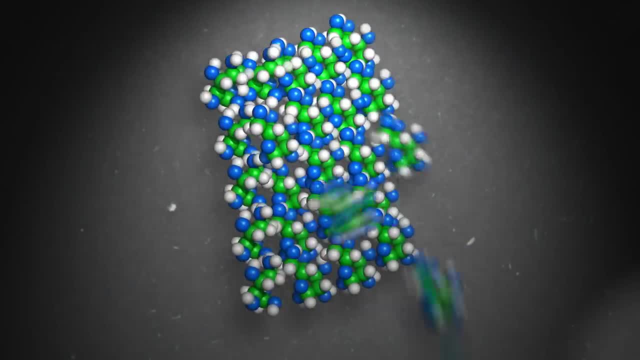 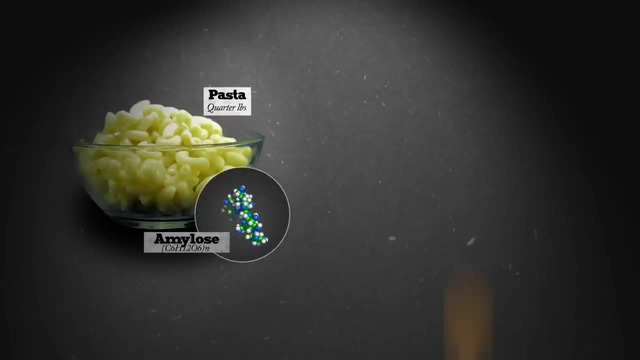 If you take a bunch of these same glucose molecules and rearrange them in a different way, you get cellulose, which is what plants are made of. So, while this piece of pasta made of amylose and this wooden spoon made of cellulose look vastly different, 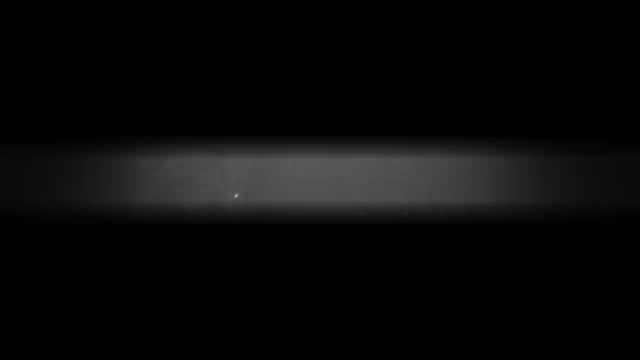 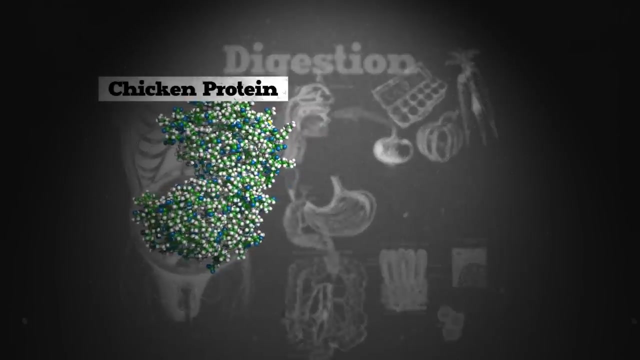 they're both essentially made of the same molecules, just stuck together differently. This type of breaking apart and recombining is what goes on when you digest food. The complex proteins found in the foods we eat, like carrots and eggs, can't be used by our bodies because we are not carrots or chickens. 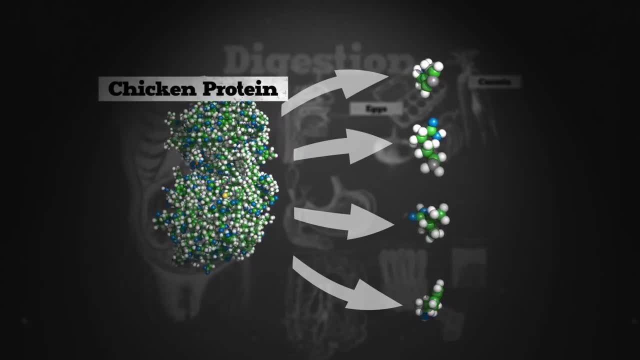 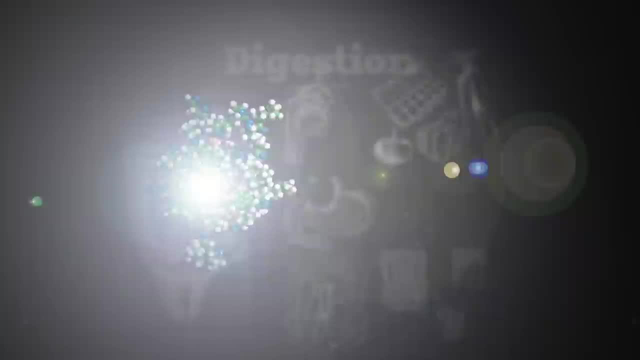 What we can use are the smaller molecules that make up these proteins, the amino acids. During digestion, our bodies break these proteins up into their amino acids, so they can be rearranged and put back together to make human proteins. But let's keep breaking bonds. 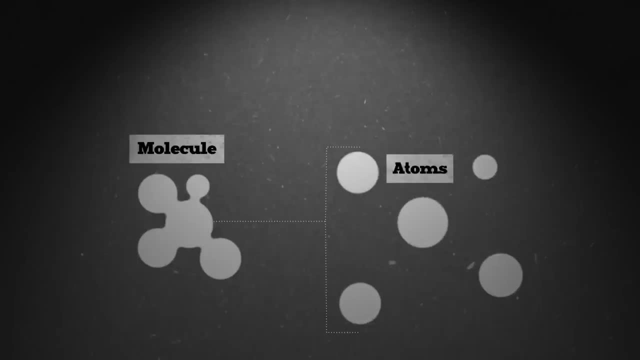 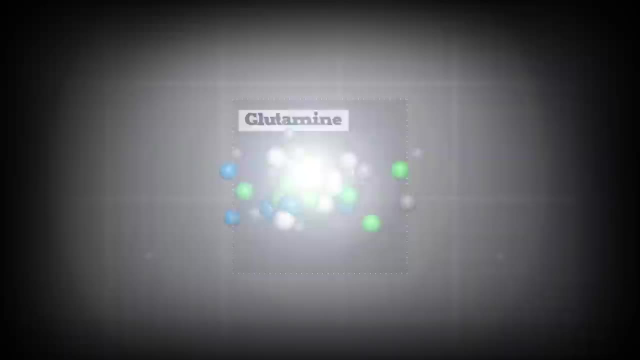 All molecules are just made up of atoms bonded together. If some molecules are building blocks, atoms are the building blocks of the building blocks, And you'll notice that with the molecules from macaroni salad, the same six types of atoms keep showing up. 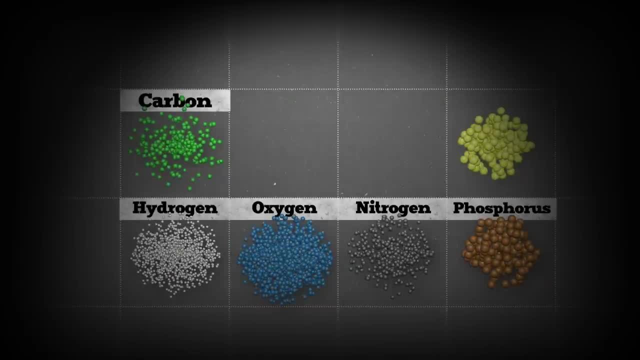 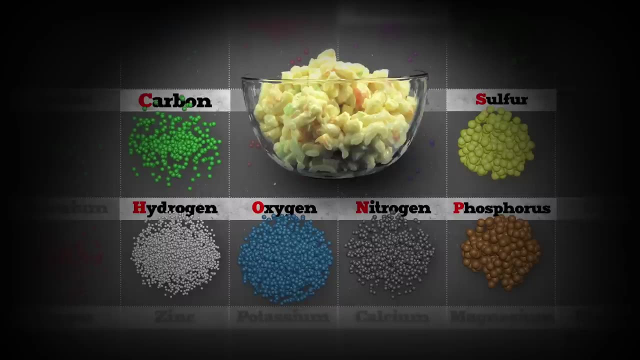 Carbon, hydrogen, oxygen, nitrogen, phosphorus and sulfur, or chomps. There's a few others, but the big six is what macaroni salad is made of. If we went a step further, we could use these same atoms. 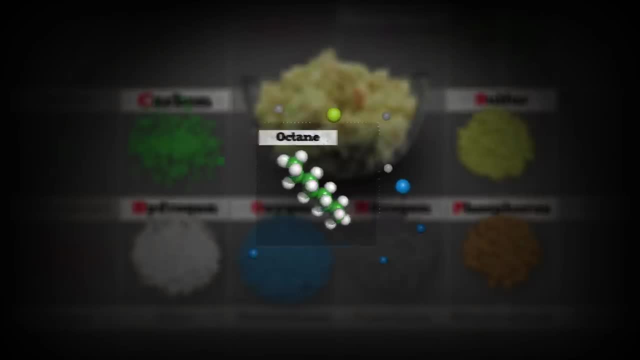 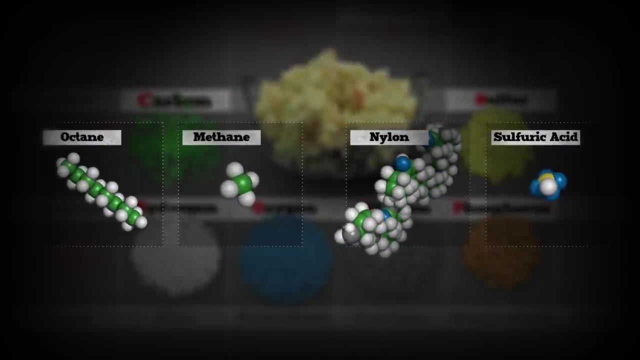 recombine them and make other stuff like gasoline or sulfuric acid, methane and nylon. It's all made from the same elements that make up macaroni salad. So, to recap, everything is made of atoms. They are the stuff that things are made of. 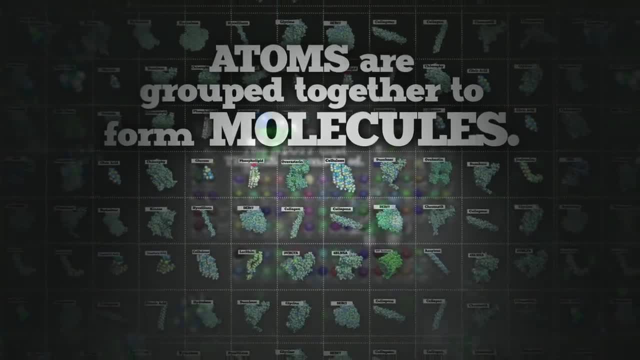 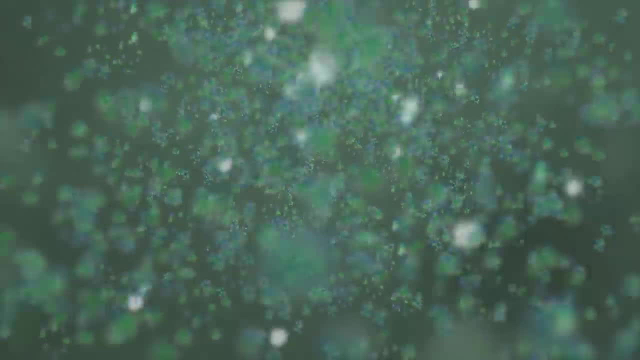 Atoms are grouped together in different ways to form molecules. These molecules are constantly being combined, broken apart and recombined. They get thrown into mixtures, separated, remixed over and over and over again. The stuff that things are made of is always in flux. 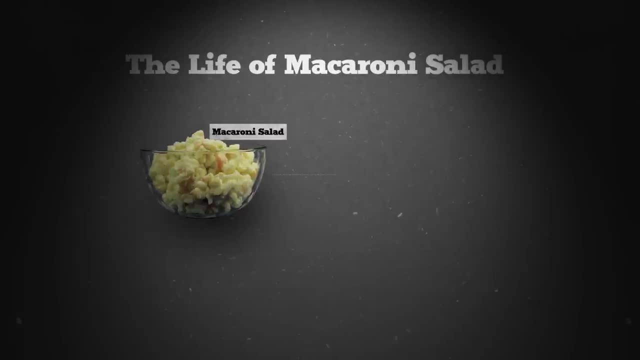 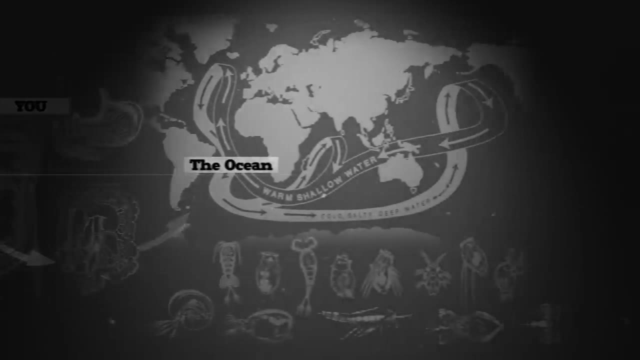 It's always changing. Macaroni salad is only macaroni salad for a short time. You eat it. some of it becomes part of you. the rest eventually goes into the ocean and gets eaten by other animals that die and after millions of years they turn into oil.